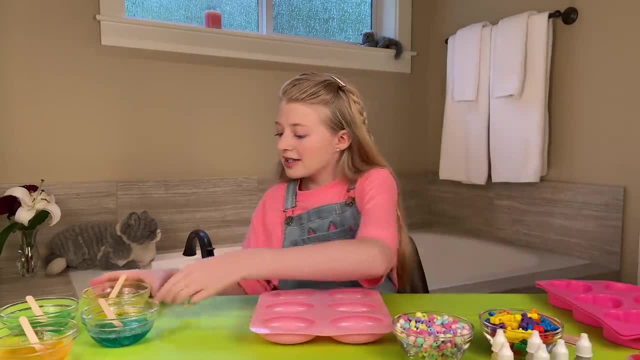 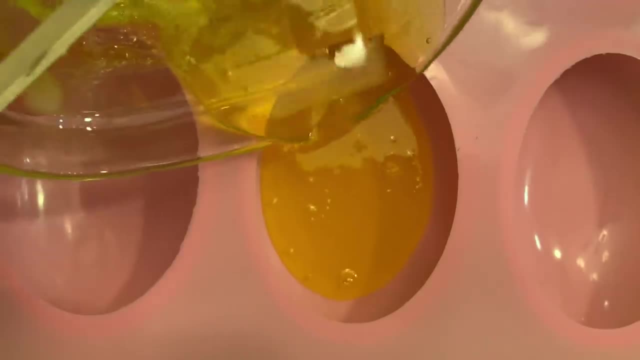 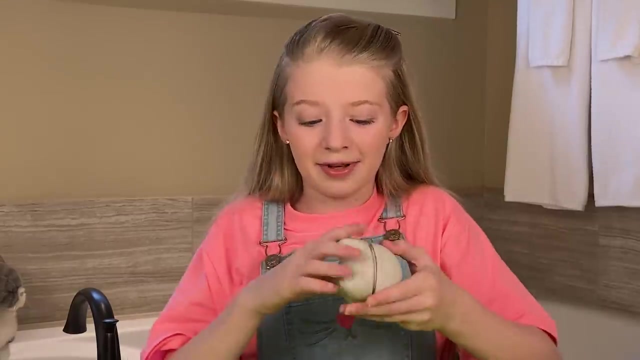 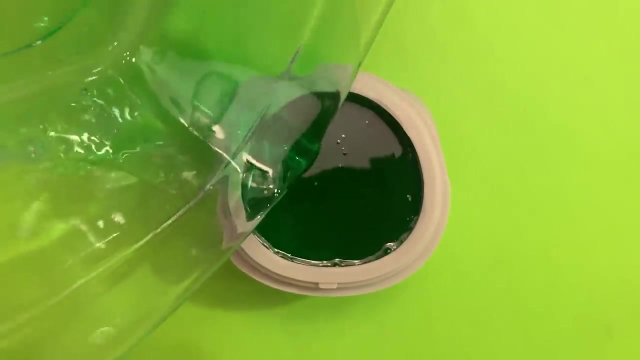 First, I'm going to do Baby Box's egg shape. Okay, Baby Box's soap looks good. Mercat, does the kitty shape. This one is gonna be cute. Okay, Okay, Okay, Okay, Okay, Okay, I want mine to be shaped like an ice pop. 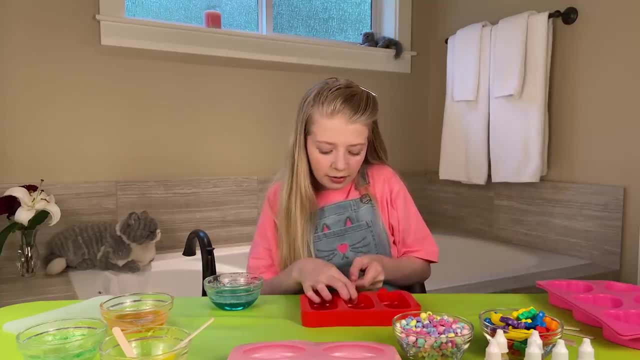 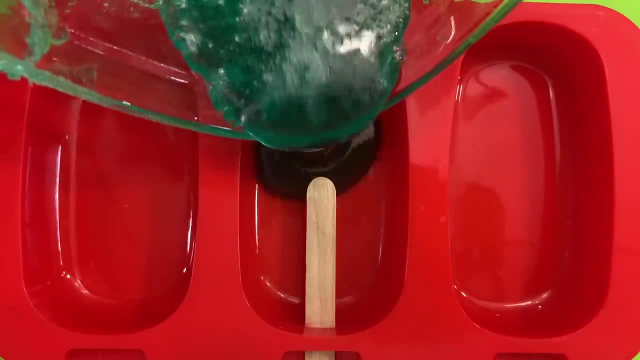 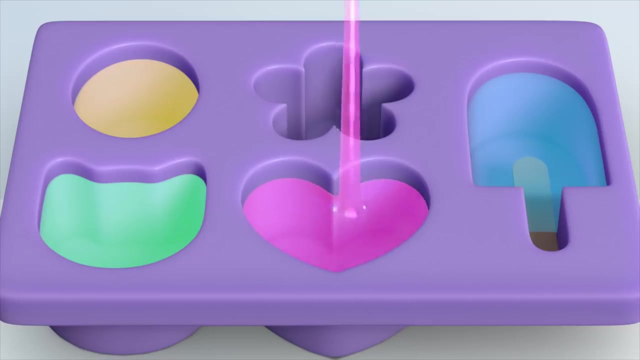 So since he did a ice pop, I'm going to put a popsicle stick in this. Now I'll put that in the middle one. I like the heart shape. Her soap kind of turned out a little orange, but I like it. 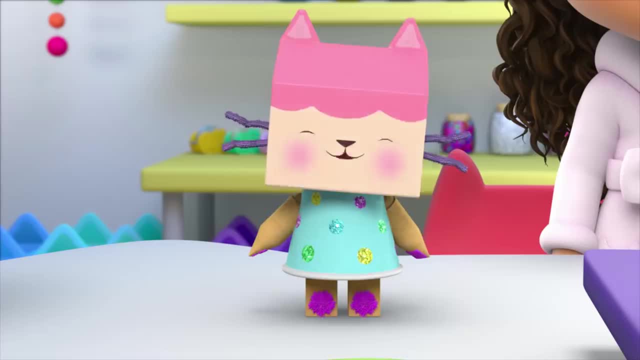 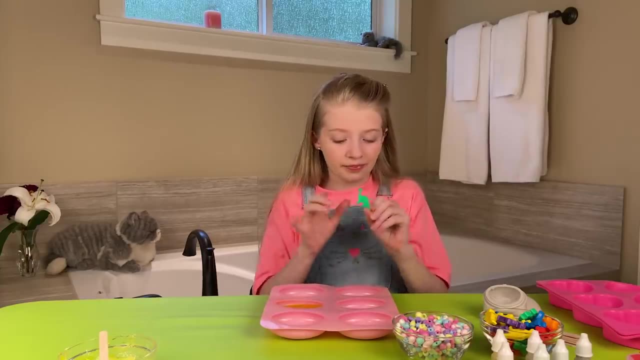 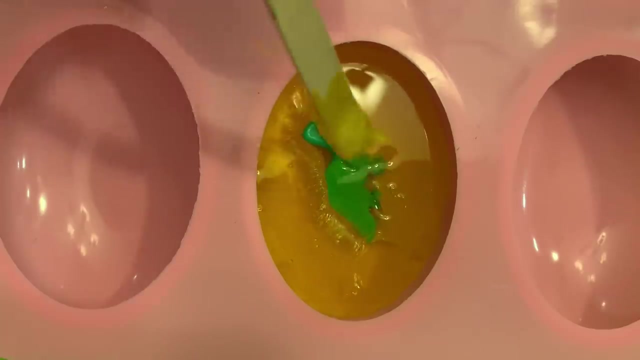 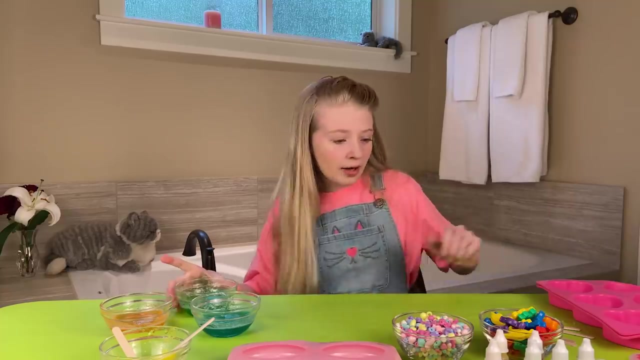 It's a pretty pinkish coral color. Now we get to pick out our super special charms. So Baby Box has a dinosaur shaped charm, So I'm gonna put that in hers. I see the perfect one for me. Now I'm going to pour this into Mercat's mold. 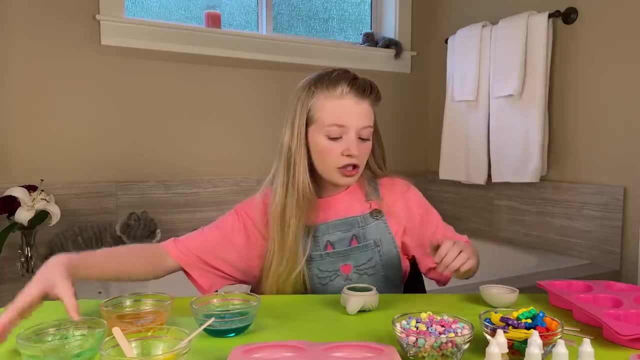 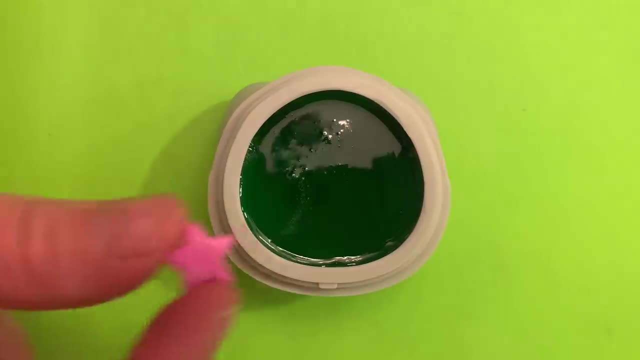 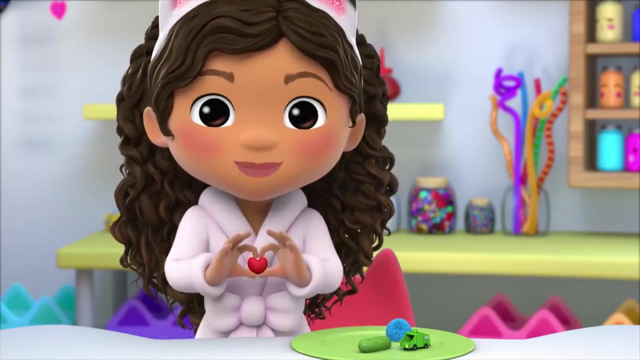 Let me just do that. She put a pink star, but I'm gonna put a couple of pink stars because I wanna make it my own. you know I love hearts, so this is my special charm. She put another heart in her heart. 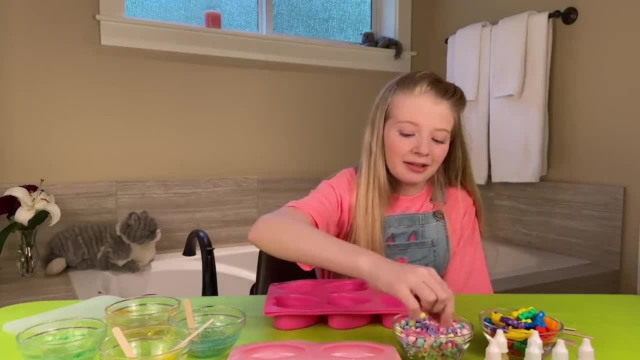 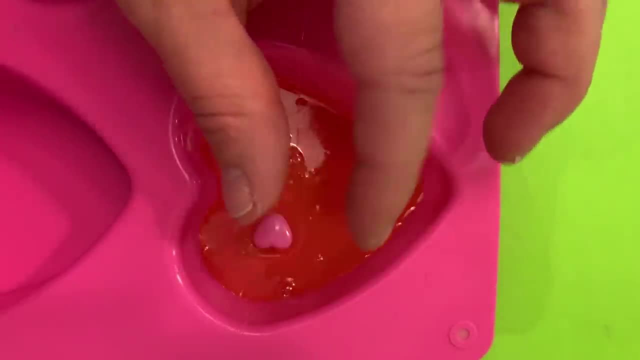 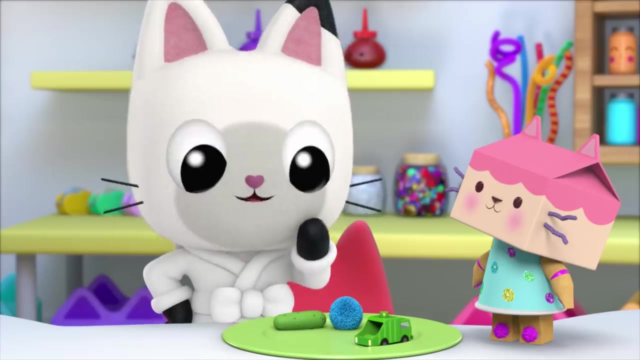 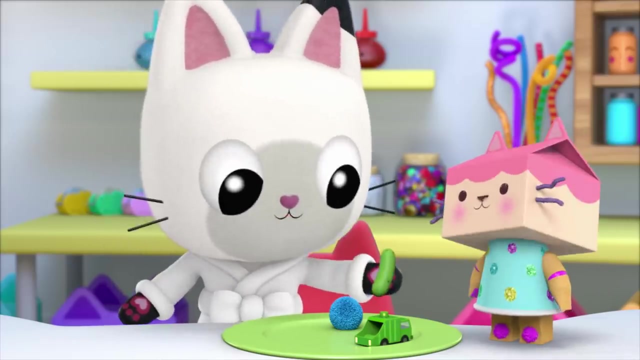 but I love stars, So I'm gonna put a lot of stars and I'll put a heart, just so it's a little like hers. For my special charm, I'm gonna pick the pickle. The pickle, Yeah, cause it's silly like me. 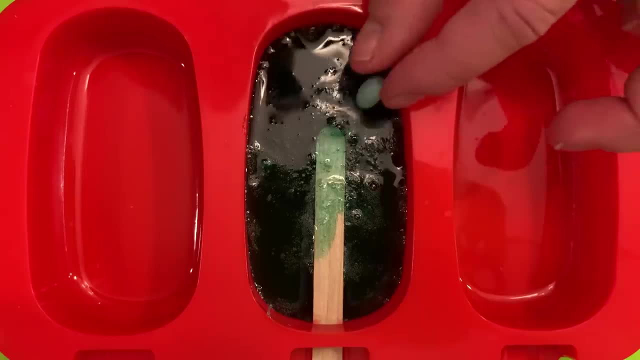 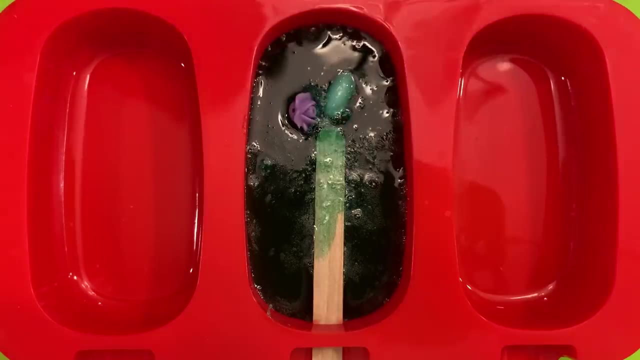 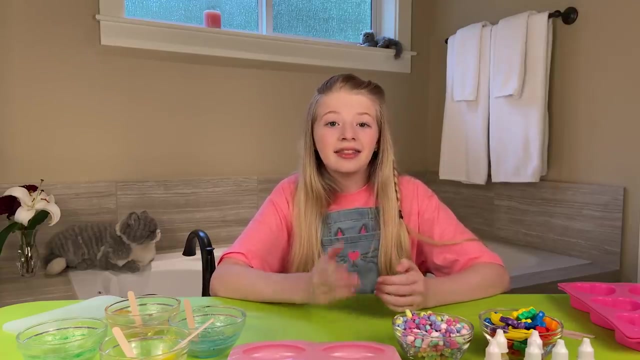 This kinda looks like a pickle, would you agree? And I'll add a flower, so the pickle's not all by itself. So now we are gonna put all of the soap molds in the freezer for 15 minutes and then we will come back and see how they turned out.